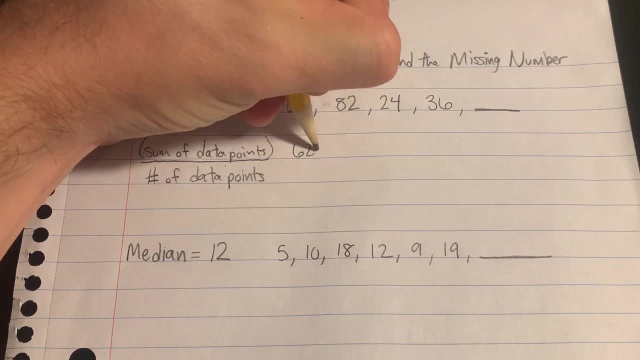 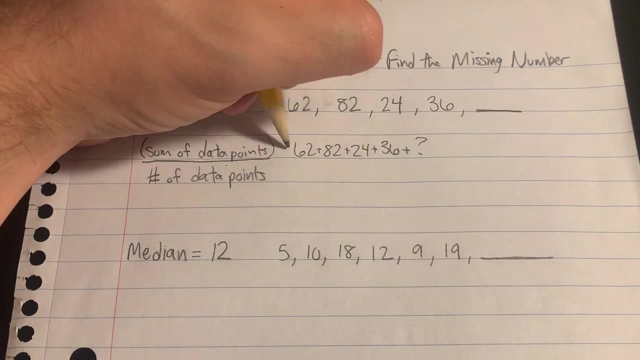 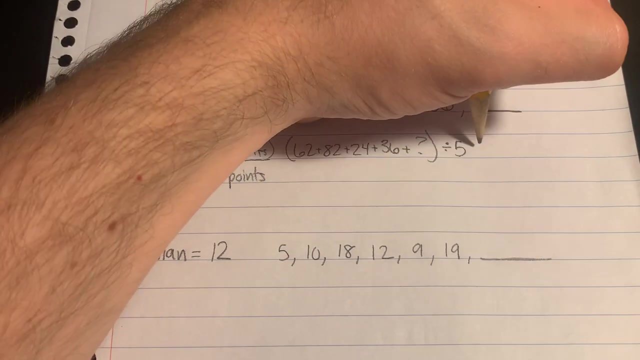 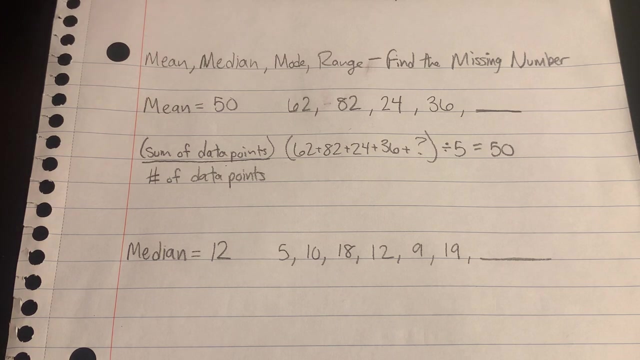 So I would have 62 plus 82 plus 24 plus 36, plus this unknown number, And then I would divide them by five, right, Because there are five of them and that's going to get me 50, okay. So if I already know what the mean is, I need to work backwards, okay. So first what? 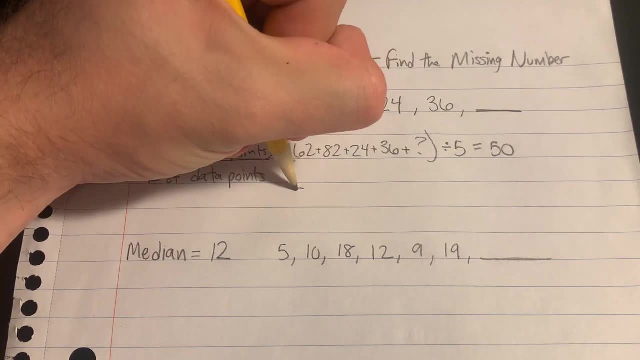 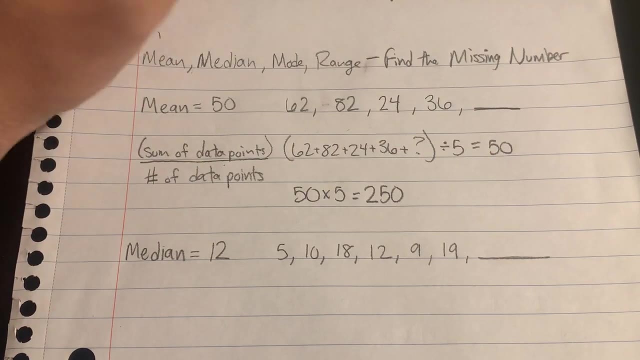 I'm going to do is: I'm going to do 50 times five. I'm going to do 50 times five, and that's going to get me 250,. okay, Then to find out what's left right. So I know that these five numbers. 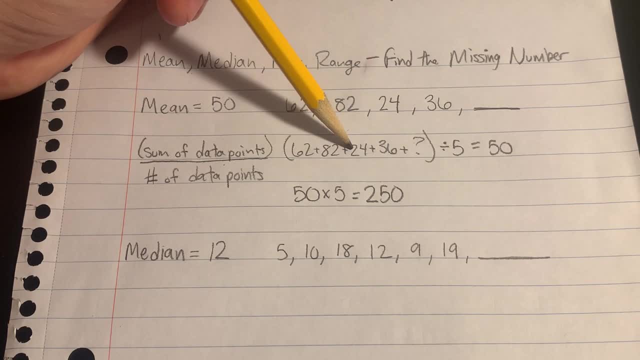 are going to add up to 250, right, 62,, 82,, 24,, 36, and that unknown are going to add up to 250.. So all I need to do is start to subtract these numbers from 250, right? So let's say I add up. 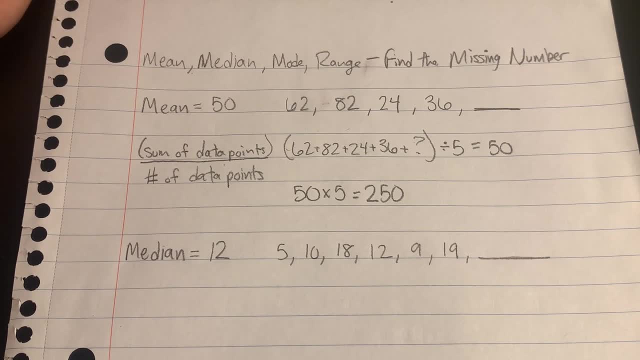 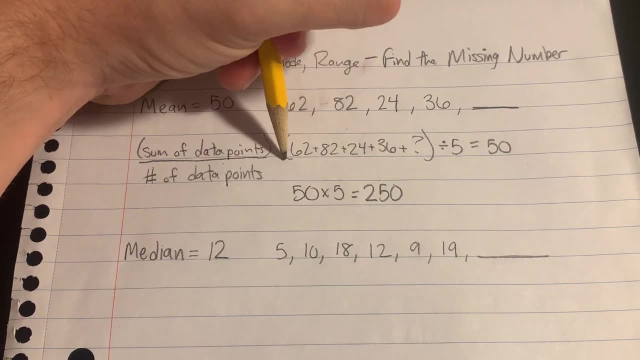 all those numbers and I have 62 plus 82 plus 24 plus 36, okay, So these four numbers together equal 204.. So then I can take 250 and add up all those numbers, right? And then I'm going to add up. 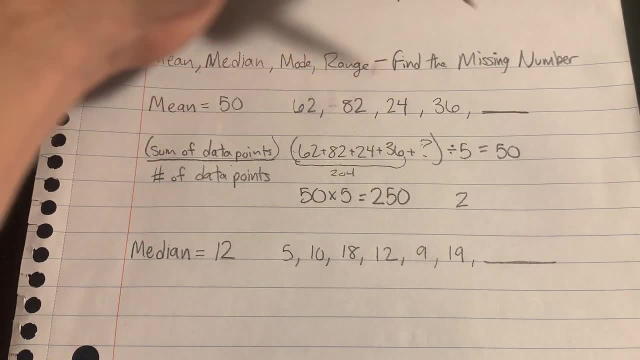 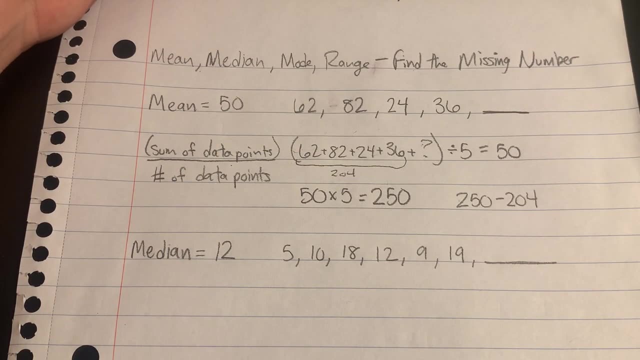 250 and subtract 204, and that'll tell me what that missing number is. So I have 250 minus 204.. 250 minus 204.. I'm sorry, I'm struggling with the mental math today, y'all, And that's going to be. 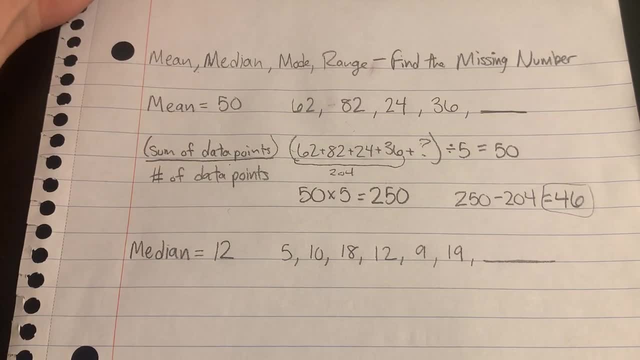 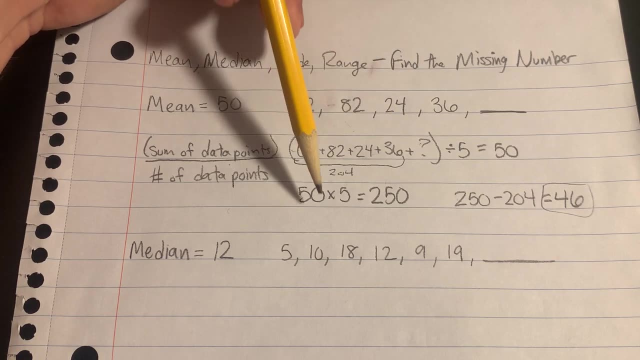 46. So my missing number would be 46,. okay, So just worked backwards, just multiplied, took the number of data points times my mean and then subtracted the data points that I already have to get 46. So that's going to be 46. So I'm going to subtract 204, and that'll tell me what. 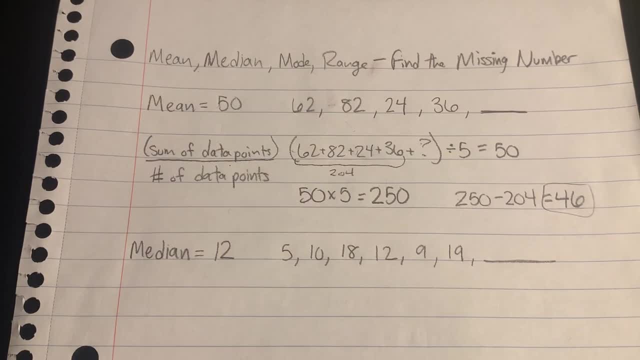 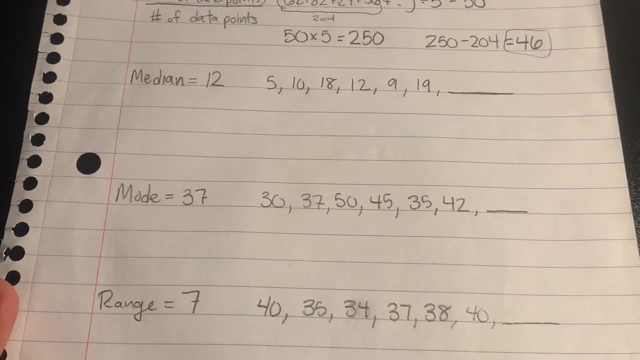 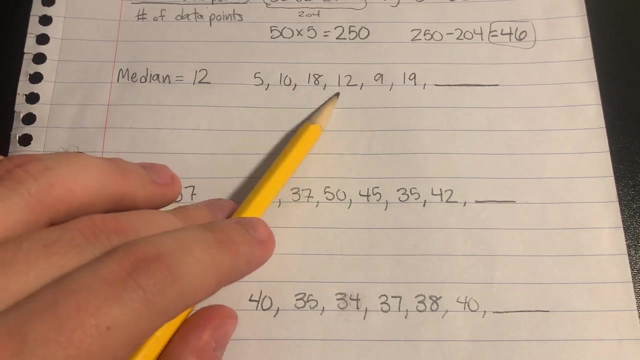 that missing number is. So again, that's the kind of the trickiest one, the one that has the most steps, The rest of them we just kind of have to reason with, okay. So let's look here at median mode and range now. So I have a data set and the median is 12.. I have 5,, 10,, 18,, 12,, 9,, 19,. 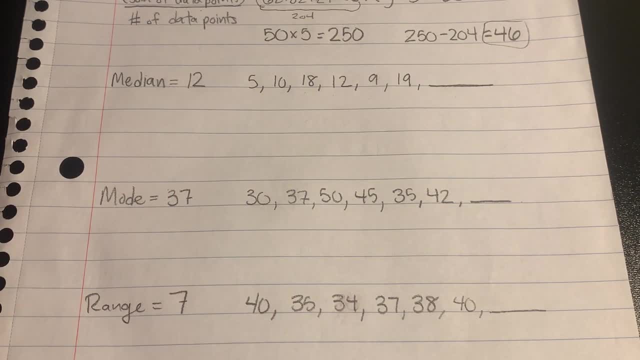 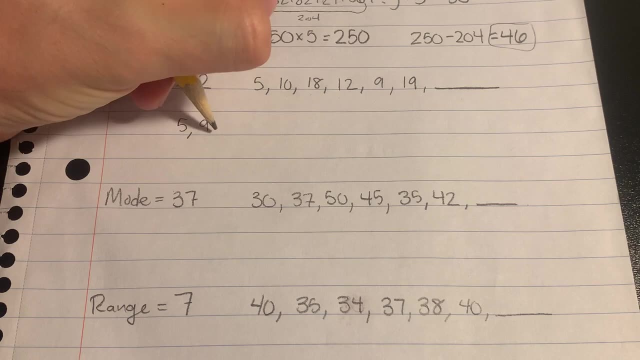 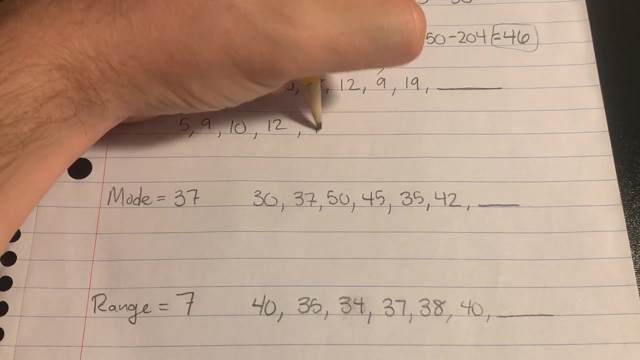 and some unknown number. The median has to be 12.. So, just like anytime I'm finding the median, I'm going to put them in order from least to greatest. So I have 5,, 9,, 10,, 12, just marking them off so I don't have duplicates. 18, and I make sure I get them all. 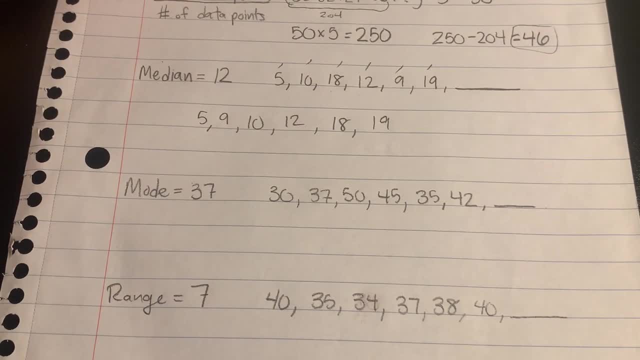 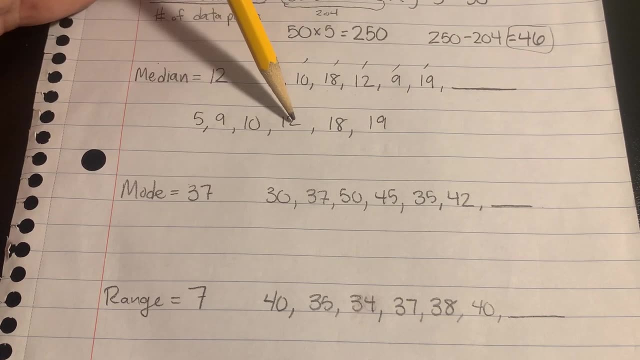 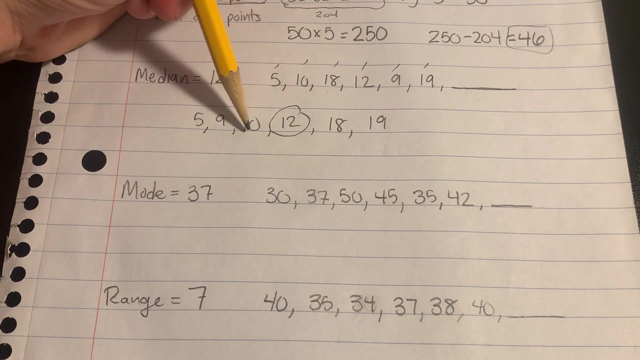 and 19.. And I have one unknown number. So I need to figure out what this unknown number could possibly be so that the median could be 12.. So I know that I need 12 to be in the middle right. 12 is my median. So that means that I'm going to have three numbers. If I have three numbers on the 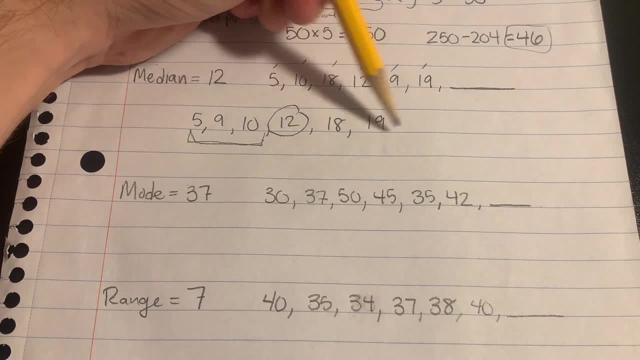 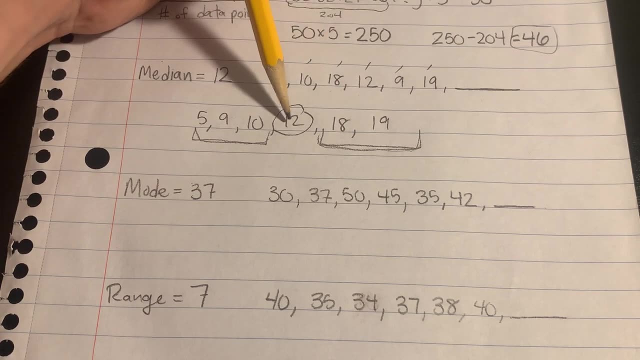 left, like I do here. right then I need to have three numbers on the right And right now I only have two. I only have two numbers on the right, So this missing number could be anything that is 12 or greater. It could. 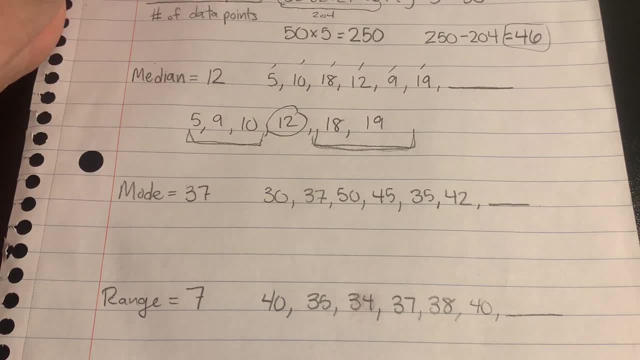 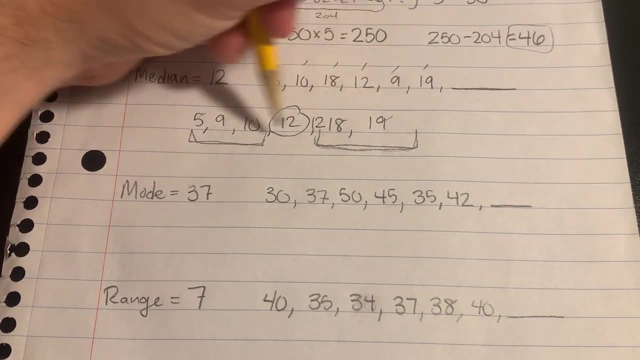 be anything that's 12 or greater. And the reason why is because if I were to put a 12 here, if I filled it in a 12, I could cross out 1, 1, 2,, 2,, 3,, 3, and I'd be left with 12, right, I could also. 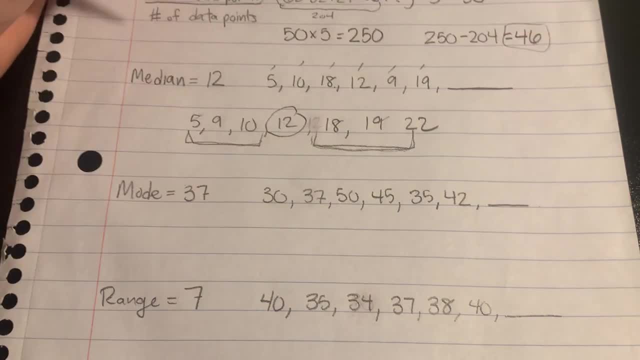 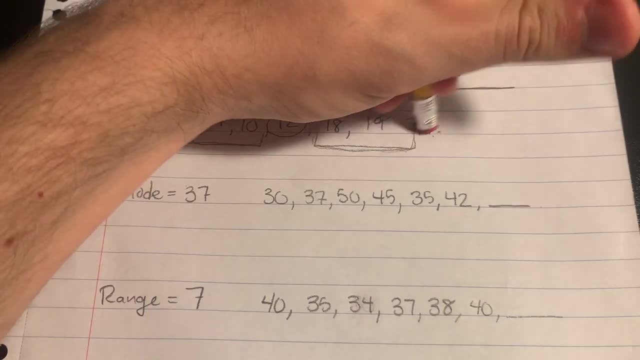 make it, I don't know- 22.. And I could put it on the outside, over here, And then it's the same thing crossing out and I'm going to end up with 12.. I could make it 15 if I wanted, And same thing. 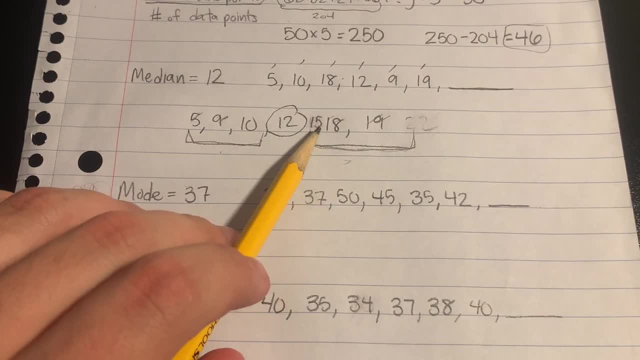 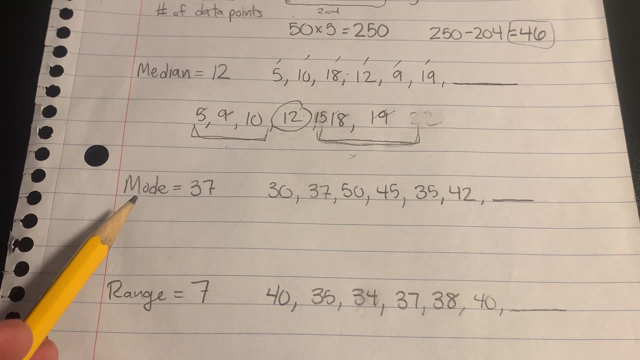 right, Anything just that's going to even out the two sides will get me a median of 12, okay, Um, let's look at mode now. So the mode is 37 for this data set And if I'm looking at the data, 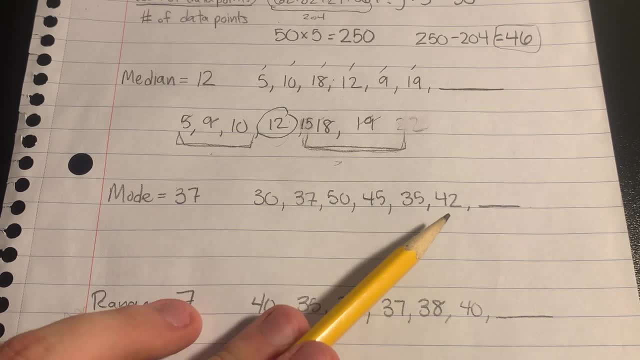 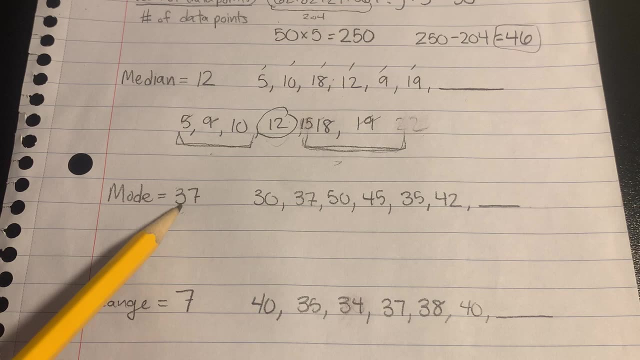 I don't have any numbers that repeat, right? Um, I do have 137. And, if I know, the mode has to be 37, right, then 37 has to be the most common number, So that missing number has to be 37, right? Just? 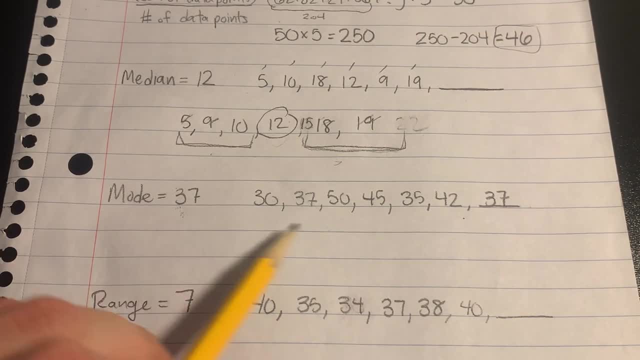 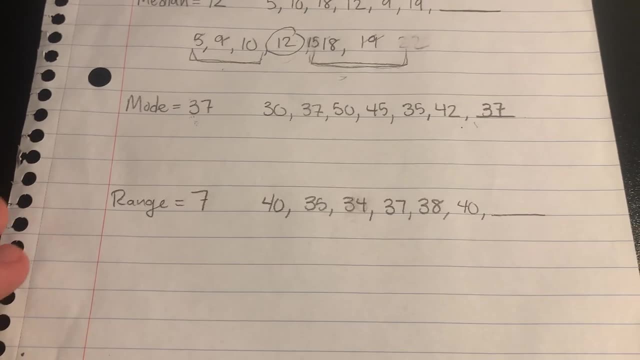 have to think about what's going to make this 37 the most common, right? Um? and in this case, adding a 37 makes it the most common. okay, Let's look at the range now. Um, if the range for a data